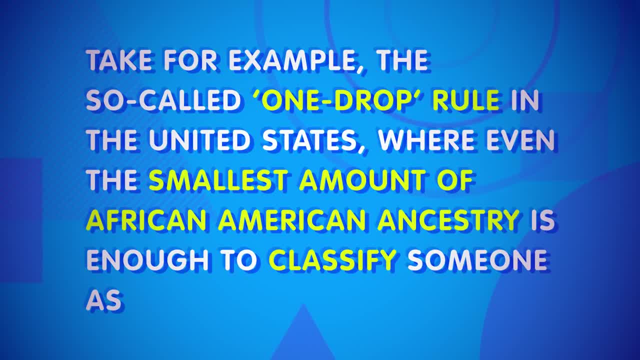 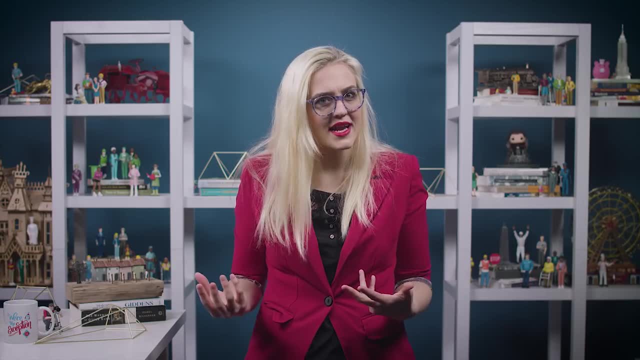 smallest amount of African American ancestry is enough to classify someone as black rather than white. The opposite, however, isn't true. Someone with one black parent and one white parent is almost never considered white. Plus, people from different places or different time periods have defined racial groups differently. 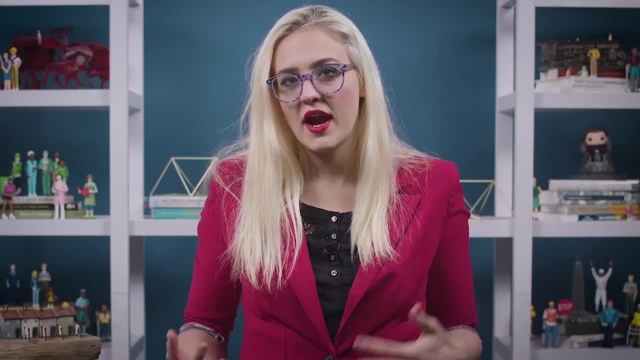 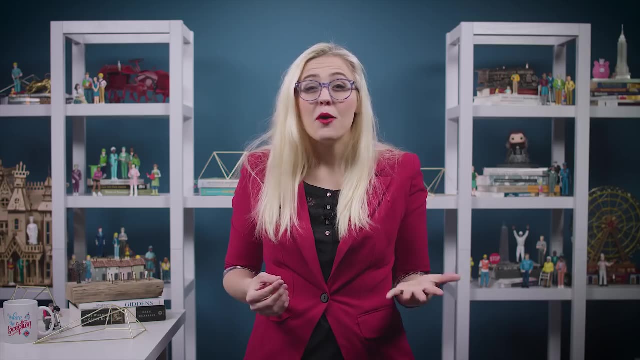 Nowadays, light-skinned people of European descent are typically considered white. in the United States, It doesn't matter whether your heritage is British or Irish or Italian or Polish or German – you're just white. But that wasn't the case a century ago. In the early 1900s, anyone who wasn't white Anglo-Saxon Protestant was considered ethnic. So, for example, if you were Italian or Irish, you weren't considered white. Likewise, today, being Jewish is often seen as an ethnicity in the United States. 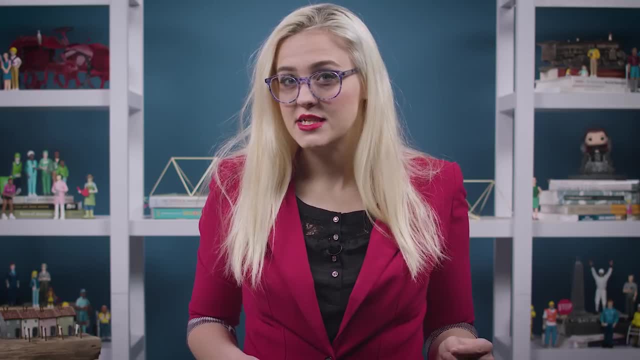 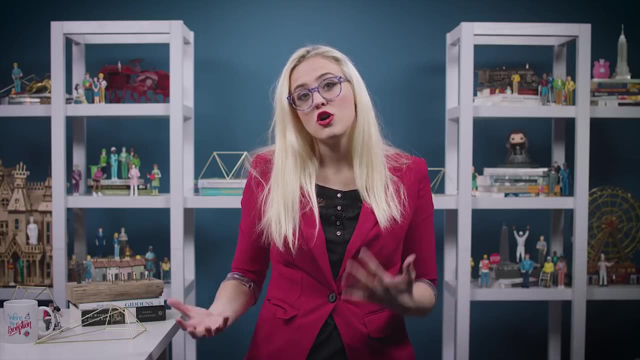 But Europeans are more likely to think of being Jewish as a race. So that raises the question – what's the difference between ethnicity and race? Well, ethnicities are socially-constructed categories, based on cultural traits that a society finds important, rather than strictly biological traits. 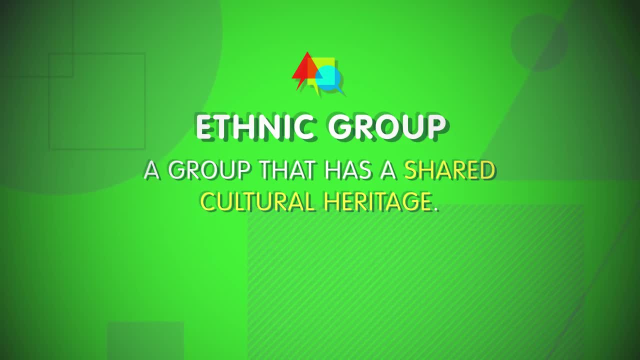 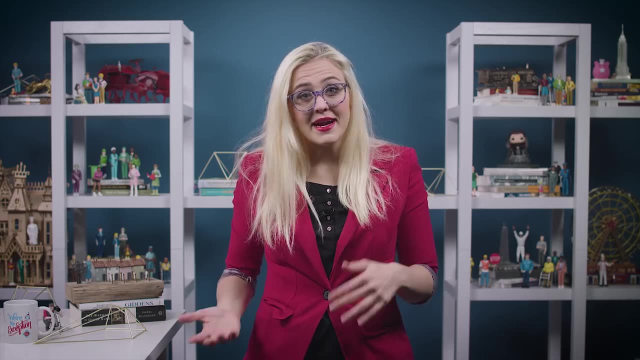 Essentially, an ethnic group is a group that has a shared cultural heritage, Language, traditions, religion – these are all types of culture that can determine your ethnic background. Two people of different races might share an ethnicity and, conversely, two people of 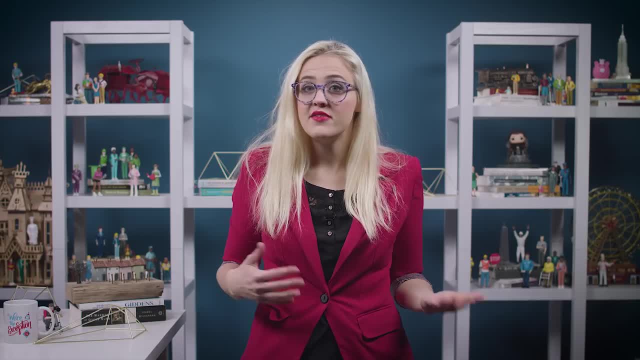 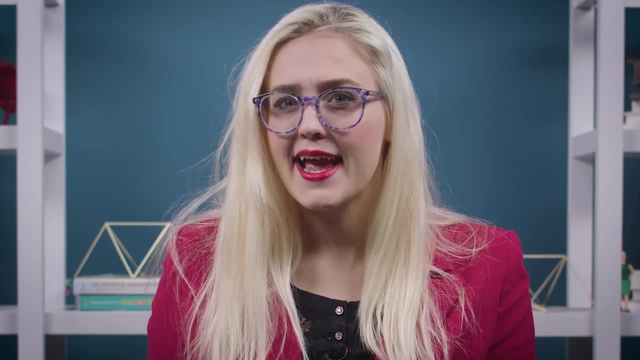 the same race might be of totally different ethnicities. Japanese and Vietnamese people are both considered Asian, but they come from different cultural backgrounds. In fact, a term that many people think refers to race- Hispanic- actually refers to ethnicity. To explore this a little more, let's go to the Thought Bubble to talk about the difference. 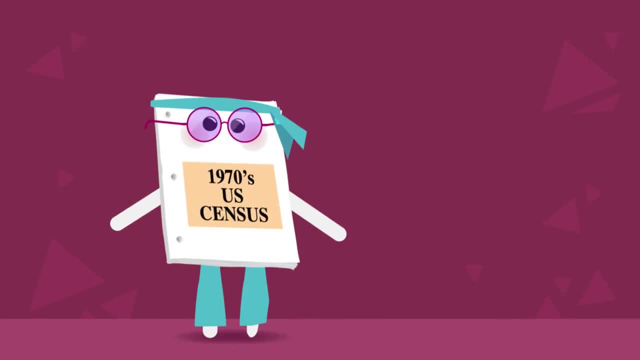 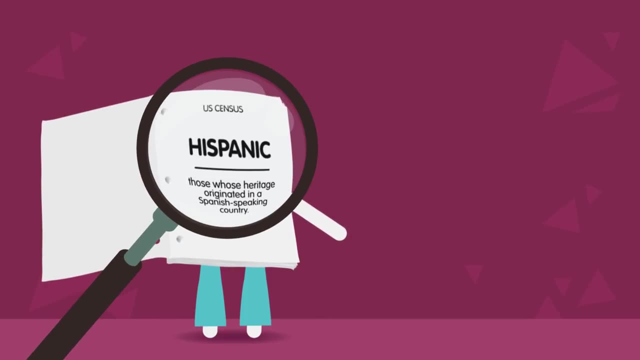 between the terms Hispanic, Latino and Latin American. The term Hispanic first appeared as a racial category in the US Census in 1970, as a way of describing those whose heritage originated in a Spanish-speaking country. Before then, the Census referred to those people as Spanish-Americans. 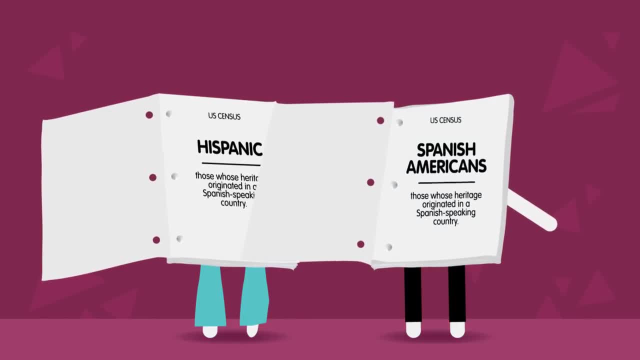 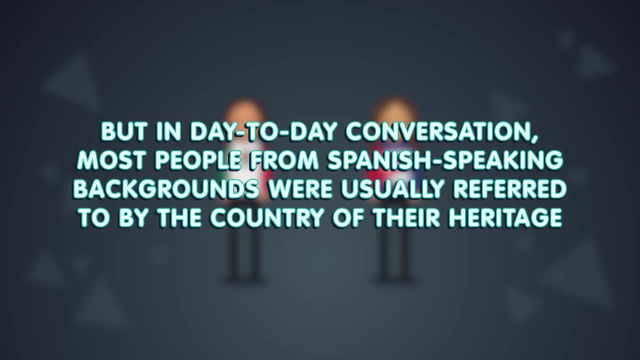 Even though tracing back their origins to Spain would mean going way, way back for many of them and for others it'd be totally inaccurate. But in day-to-day conversation, most people from Spanish-speaking backgrounds were usually referred to by the country of their heritage, like Mexican-American or Cuban-American. 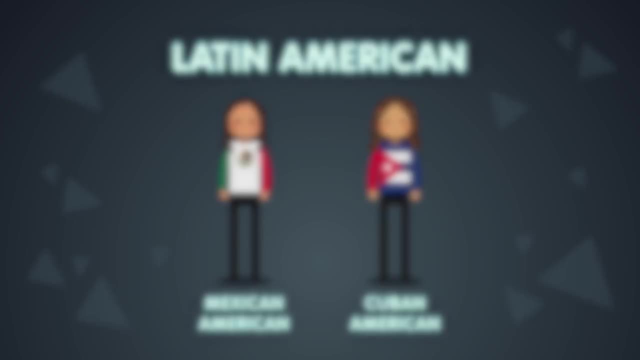 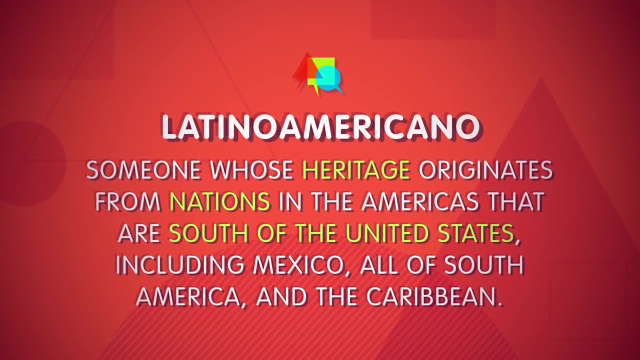 or sometimes more broadly, as Latin American. This last term is also where we get the word Latino and the degendered Latinx. It's a shorter version of the Spanish word Latinoamericano, and it refers to someone whose heritage originates from nations in the Americas that are south of the United. 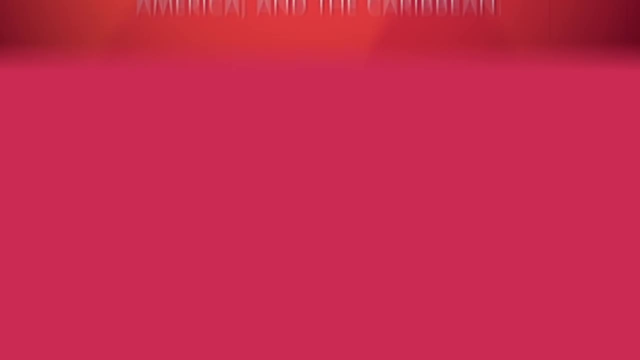 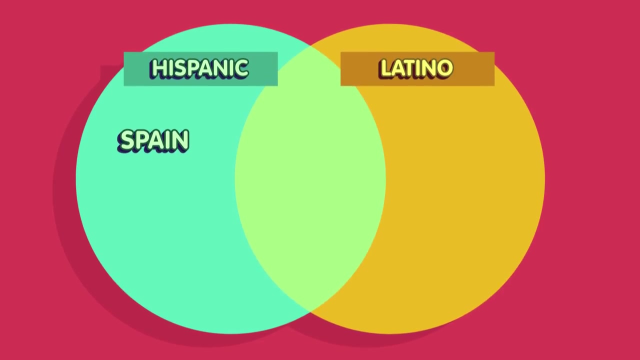 States, Mexico, all of South America and the Caribbean. Now, not all Hispanics are Latino. Being from Spain, for example, makes you Hispanic but not Latino, and not all Latinos are Hispanic. Brazilians speak Portuguese, meaning that they are not considered Hispanic. 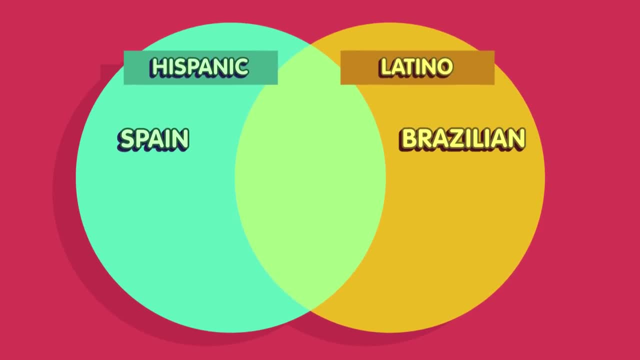 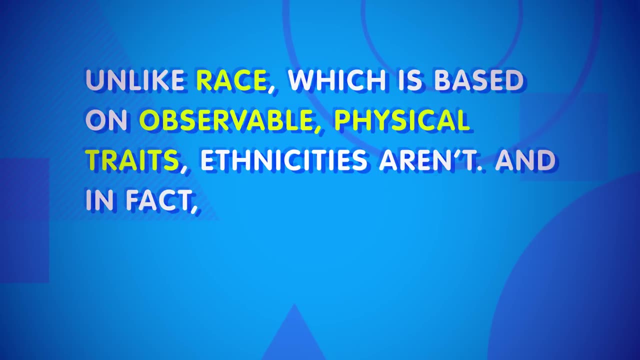 But regardless of which term you're using- Hispanic or Latino- neither of these distinctions are based on physical appearance, Unlike race, which is based on observable physical traits. ethnicities aren't, And in fact, two people of the same ethnicity can be entirely different races. 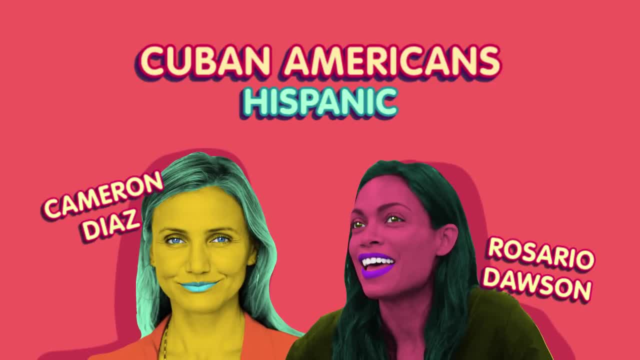 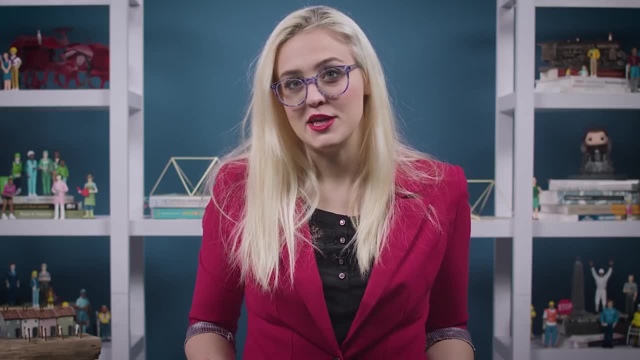 For example, both Cameron Diaz and Rosario Ramos are Hispanic And Rosario Dawson are Cuban-Americans, which means they are both Hispanic, But Cameron Diaz is white and Rosario Dawson is black. Thanks, Thought Bubble. Though race is more commonly used by society as a way to organize people and distribute. 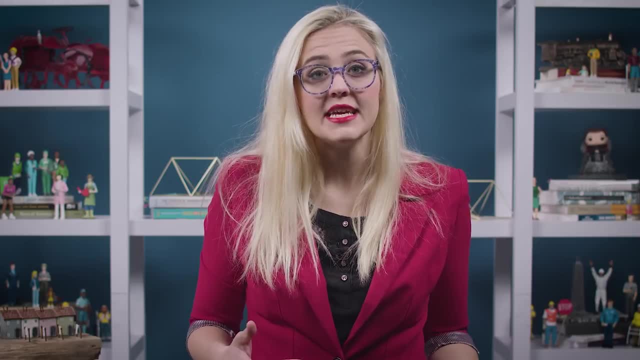 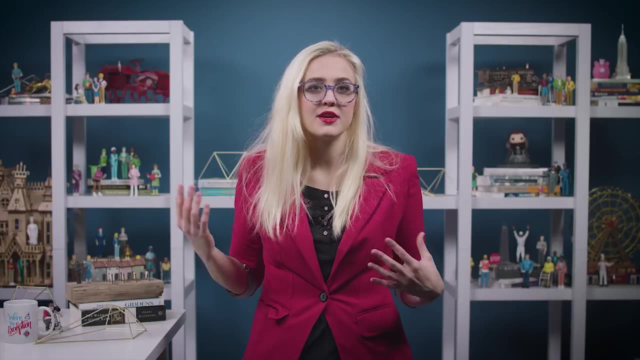 power. both race and ethnicity play a role in how people are perceived and therefore, the opportunities that are available to them. A person's race influences a whole host of social outcomes, from their education to their income, to their experiences with the criminal justice system. 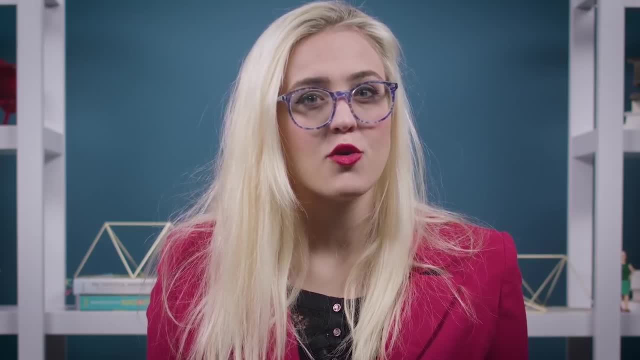 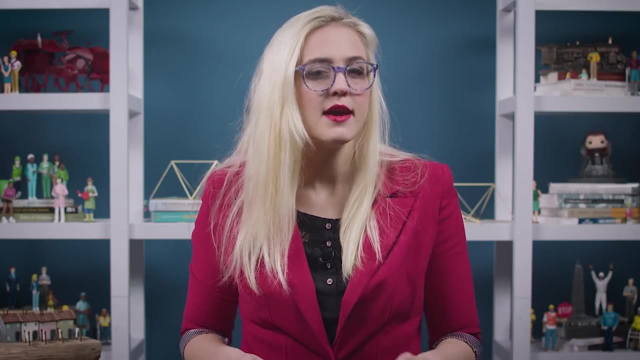 But which races or ethnicities are advantaged or disadvantaged depends on when and where we're talking about. For example, in the United Kingdom there's been a lot of unrest about immigration from Eastern Europe, especially Poland. Incidents of hostility and violence against Polish immigrants have increased in the wake. 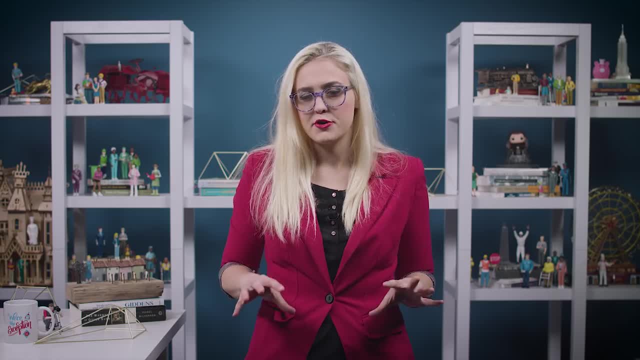 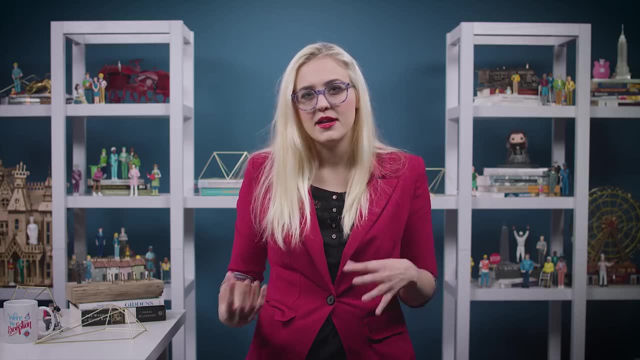 of the UK's exit from the European Union. But while Eastern Europeans are considered an ethnic minority in the UK, people in the US are much more likely to think of Eastern European immigrants as just white. They're not thought of as a minority, And that's because what constitutes a minority is more complex than you might think. 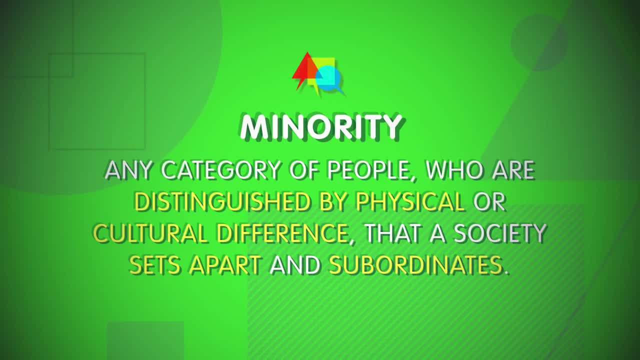 Sociologists define a minority as any category of people who are distinguished by physical or cultural differences. They are a minority of the group that is considered a minority, and they are considered a minority because of the difference that a society sets apart and subordinates. 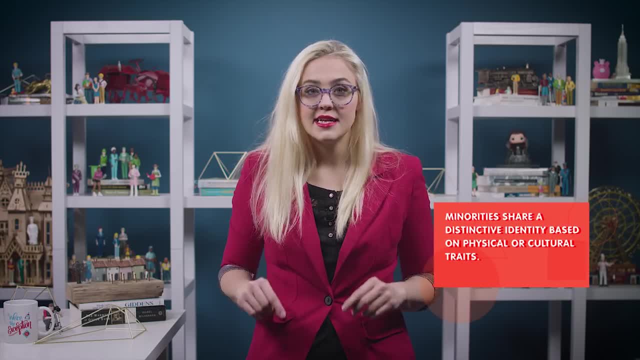 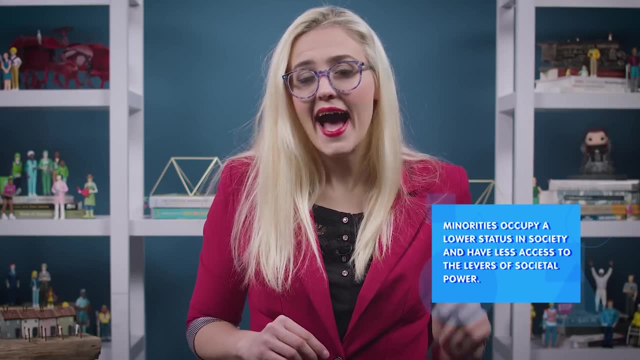 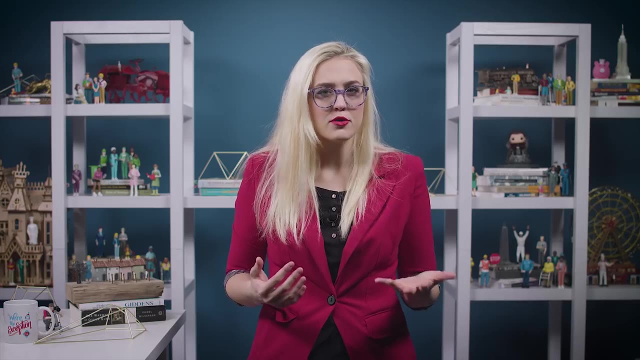 Now notice that there are two important parts of that definition. First, minorities share a distinctive identity based on physical or cultural traits. Second, minorities occupy a lower status in society and have less access to the levers of societal power. Notice how that definition doesn't say anything about the size of the group. 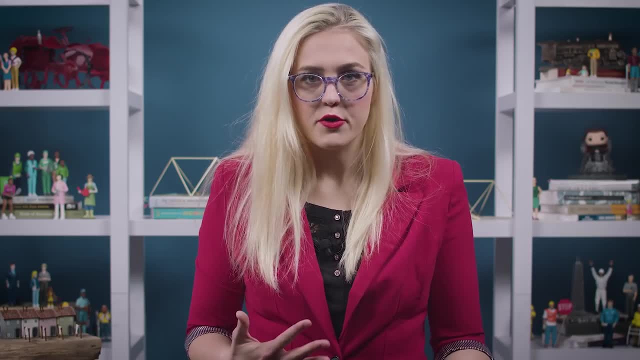 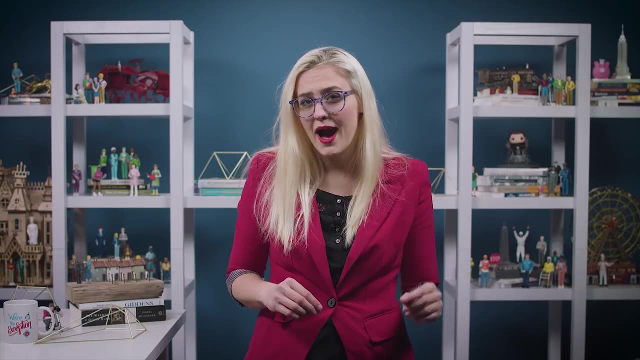 In sociology, a minority group's relative size isn't important. For example, women are considered a minority even though they make up about 51% of the United States. The majority group's relative size can still be a majority in terms of power. 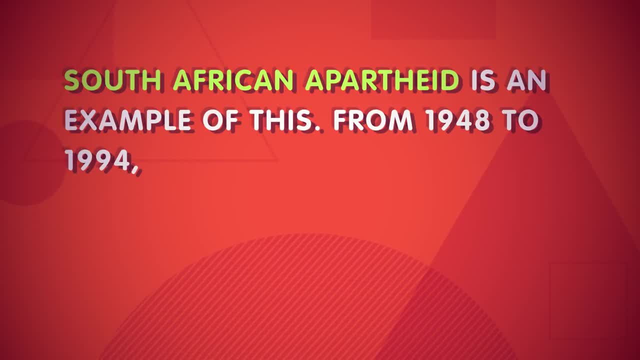 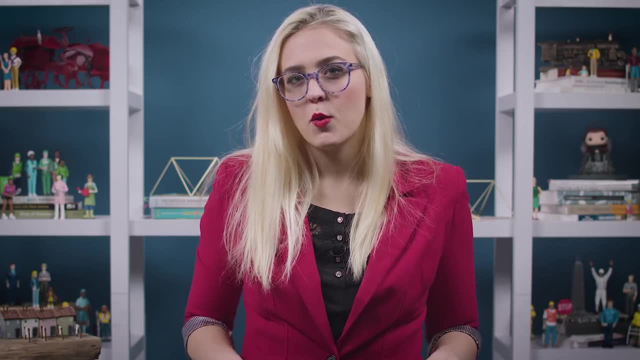 South African Apartheid is an example of this. From 1948 to 1994, a white minority maintained a system of racial segregation and discrimination against black South Africans. Right now, non-Hispanic whites are the majority group in the United States in terms of sheer. size, making up 61% of the US population, But that's rapidly changing. As of 2015,, babies of color being born now outnumber non-Hispanic white babies, and five states are already minority-majority states: California, Texas, New York, New York and New York. 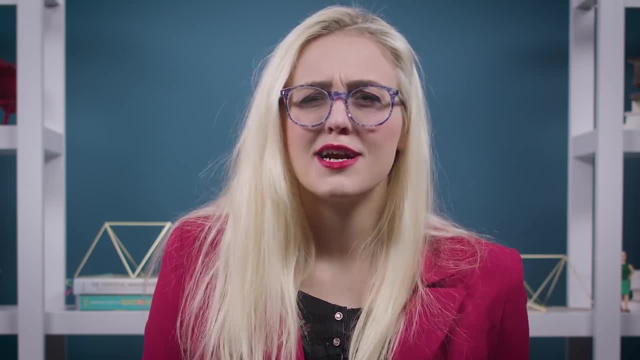 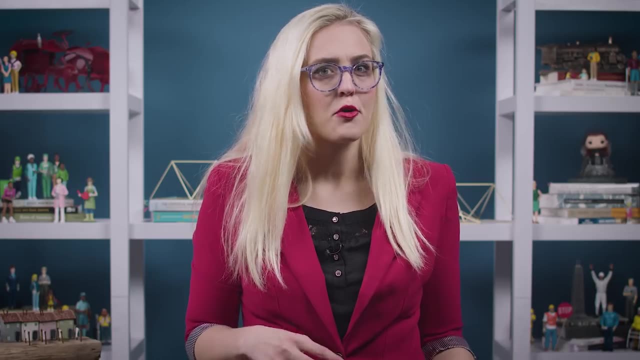 California, Texas, New York and New York, New Mexico, Nevada and Hawaii. How can a state or country be minority-majority? Isn't that like an oxymoron? Well, for one thing, even if non-Hispanic white Americans no longer make up more than. 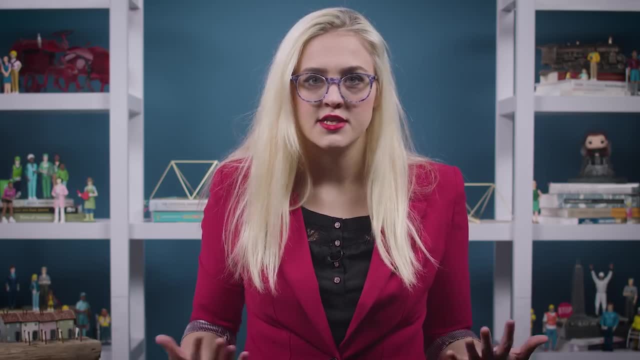 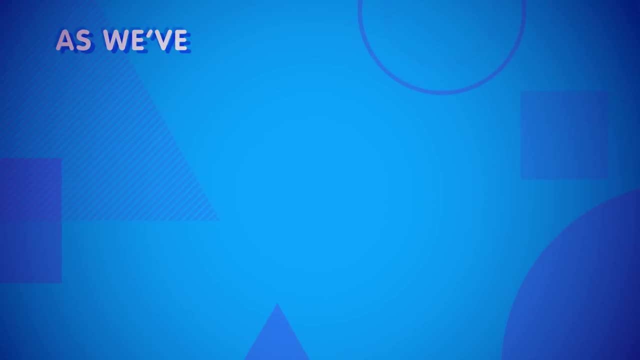 half of the country. they'll likely remain a larger group than any other single race. But also to be a minority in the sociological sense of the word, a group must be in a position of disadvantage And, as we've discussed many times before, non-Hispanic white Americans tend to have. 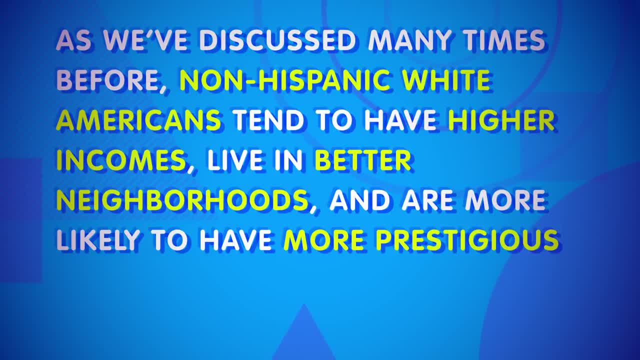 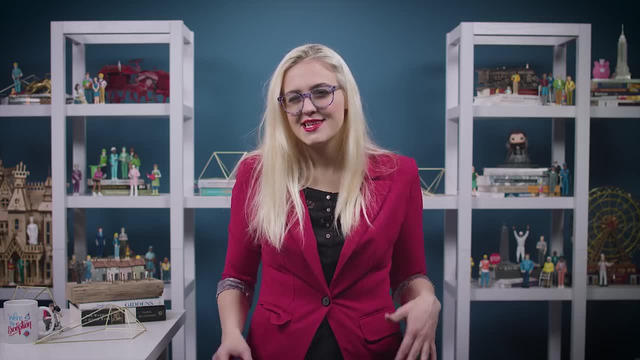 higher incomes, live in better neighborhoods and are more likely to have more prestigious jobs and better educations than non-Hispanic white Americans. But before we can make comparisons between different racial groups in the US, we should talk about the races that make up the United States. 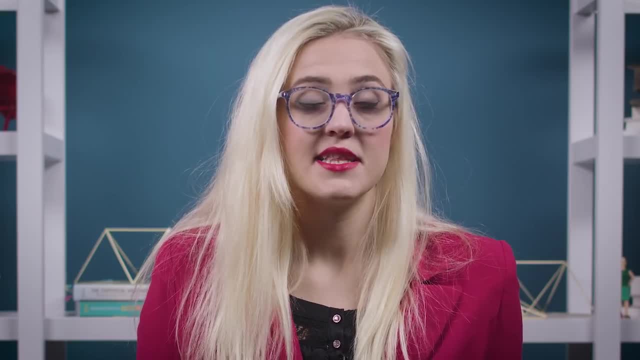 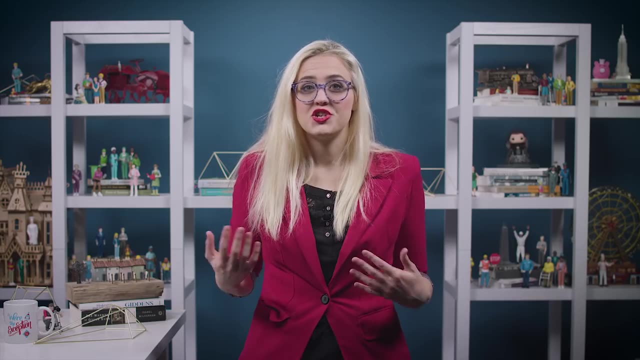 The US Census uses six different categories of race when collecting data about the demographics of the country. White refers to anyone who reports their origins as being from Europe, the Middle East or Northern Africa. So Irish, German, Italian, Lebanese, Iranian, Moroccan – they're all ethnicities that 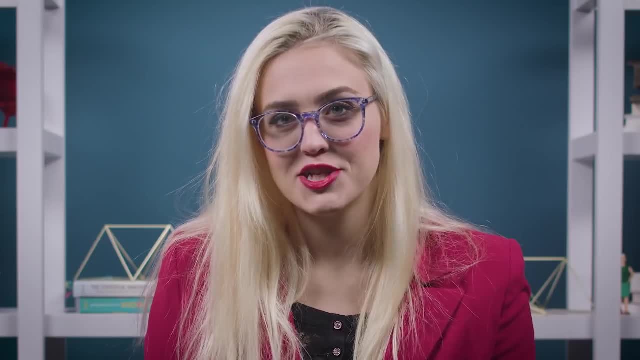 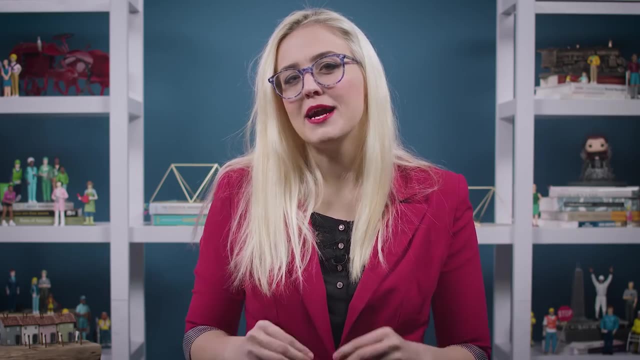 go under the heading of white. Yes, you heard me right. people of Middle Eastern descent are categorized as white by the census, Even if they often aren't treated as if they're white. Why? Well, what's now become known as white originates from a term to refer to people of Indo-European. 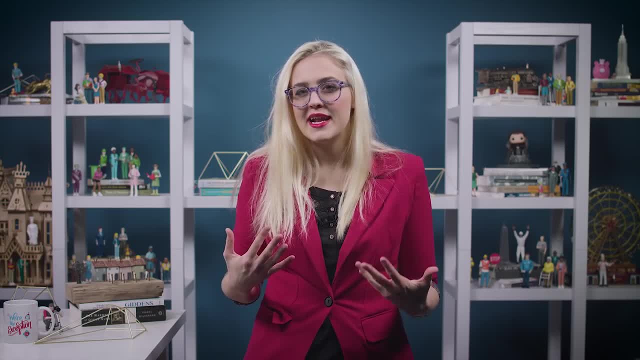 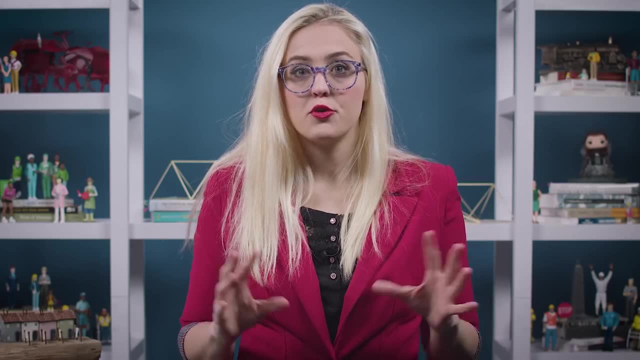 descent: the Caucasian race. The term Caucasian started as a reference to the Caucasus Mountains, which run through the modern-day countries of Russia, Georgia, Armenia and Azerbaijan. Back when race was understood as a purely biological phenomenon, everyone from Europe all the way down to India was lumped into one Caucasian group. 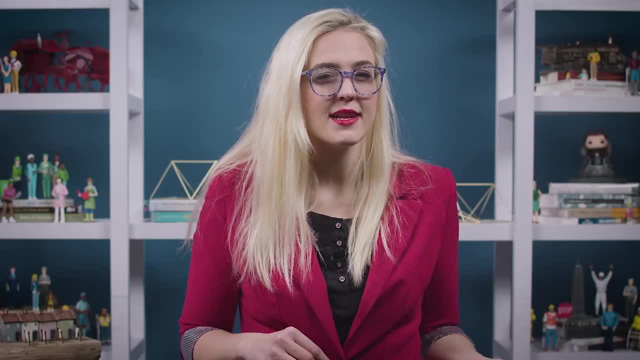 So yesterday's Caucasian contained most of the people who count as today's white, but also captured groups that nowadays get less than 50% of the population. That's a lot, And that's because they're labeled as Asian, such as Indians or Pakistanis. 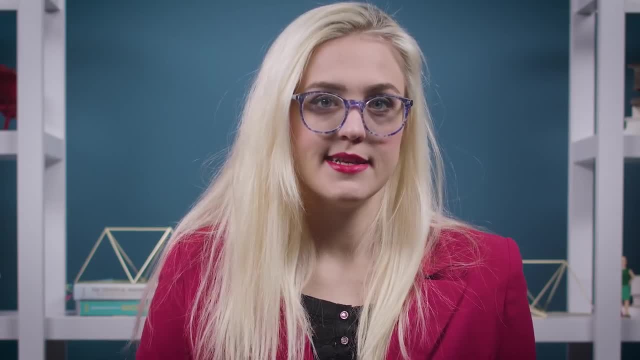 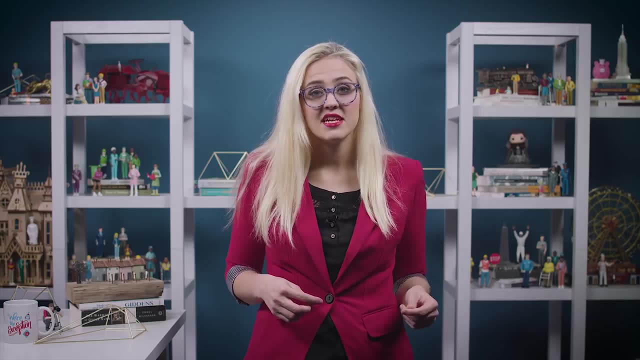 Now many Hispanic Americans are also counted as white in the census. Hispanic is considered an ethnicity, not a race, for census purposes. So in the 2010 census, 52% of Hispanic Americans identified themselves as white, while 36.7%. 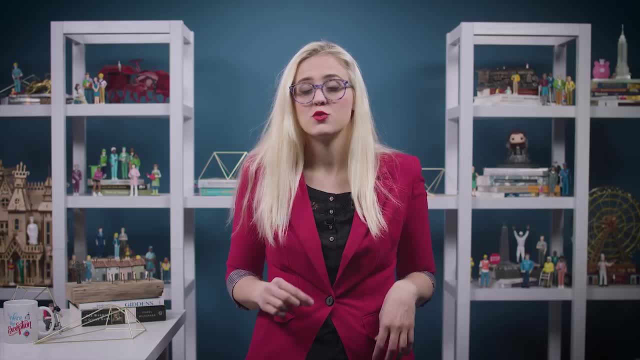 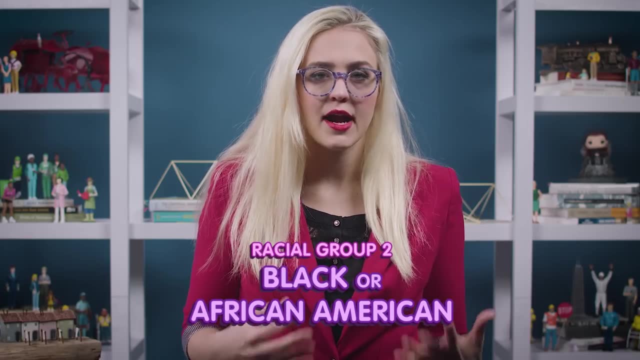 identified themselves as some other race, And smaller percentages identified themselves as one of the other racial groups. Black or African Americans are the second largest racial group in the United States and are defined as individuals with African heritage, including those who are Afro-Caribbean. 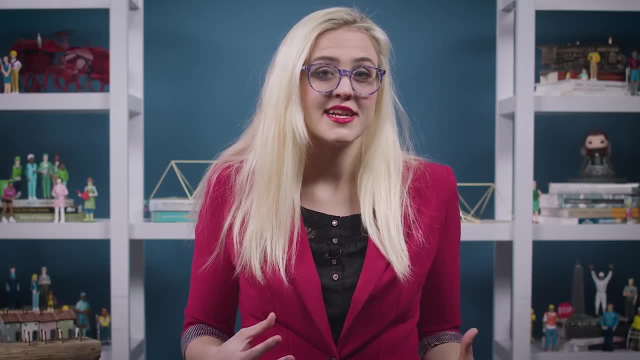 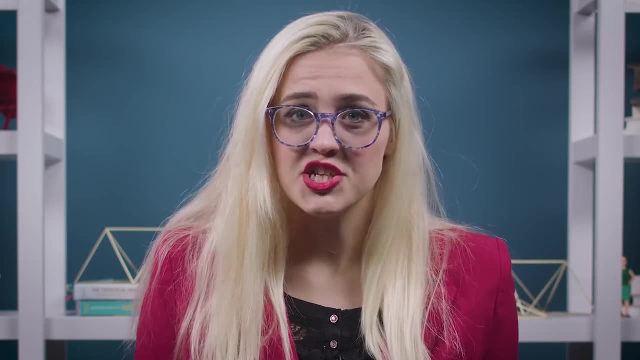 Since many African Americans' ancestors were forcibly brought to the United States as slaves, the countries that their ancestors originated from are often unknown To this day. the remnants of slavery in the southern plantation systems can be seen in the geographic distribution of black Americans around the country. 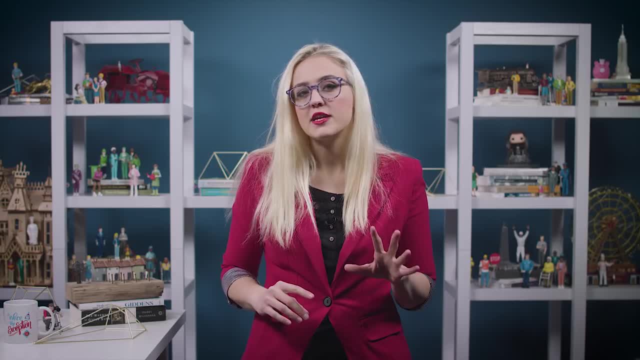 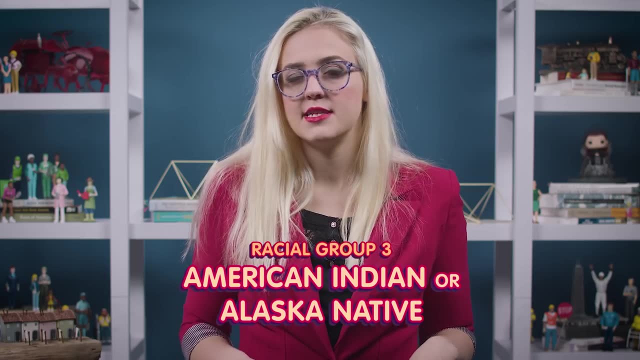 Though many black Americans moved to northern cities during the Great Migration of the early 20th century, most remained in the south, in a region that has come to be known as the Black Belt of the United States. The third racial category used in the census is American, Indian or Alaska Native, which refers to anyone whose origins are indigenous to the contingent of the African people. 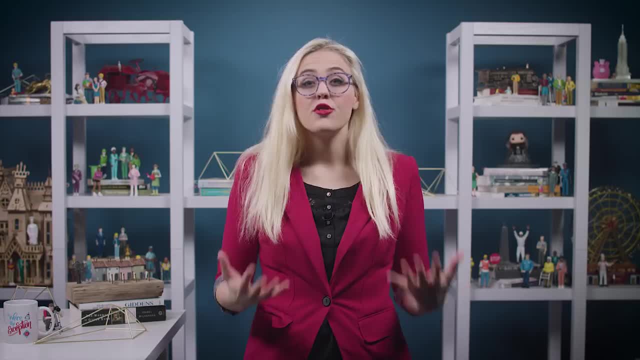 The second racial category used in the census is American Indian or Alaska Native, which refers to anyone whose origins are indigenous to the contingent of the African people indigenous to the contiguous United States and Alaska, Though Native Americans numbered in the millions when Europeans first arrived in the 15th century. 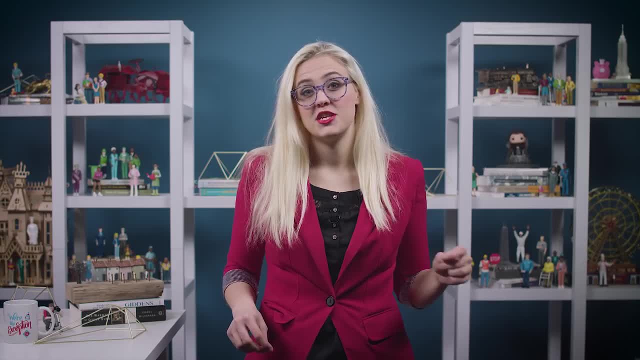 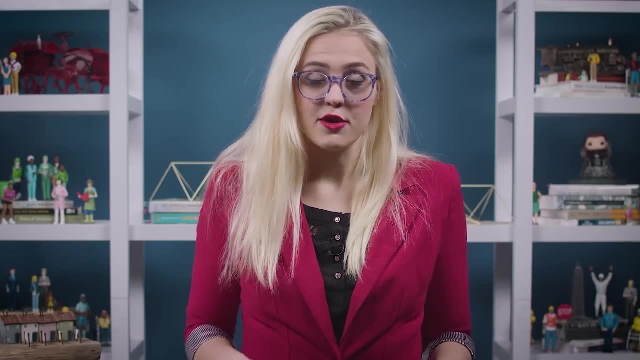 today, they control only 2% of the country's land area, make up just 0.2% of the US population and remain severely disadvantaged in terms of access to education and income. The fourth census category for race- Asian- refers to origins in Eastern Asia- Southeast. 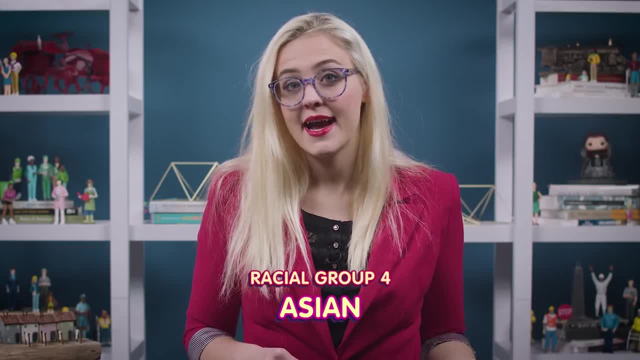 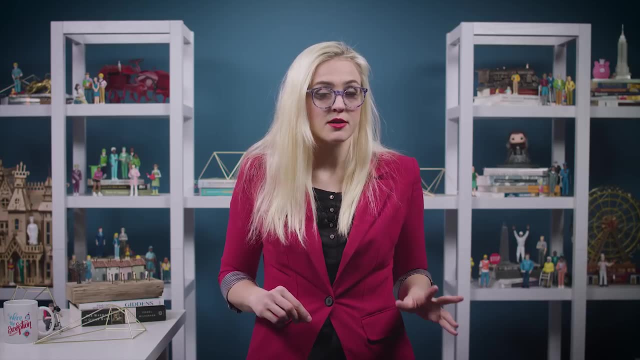 Asia or the Indian subcontinent, including China, India, Japan, Pakistan, the Philippines and Vietnam. This subgroup of Asian Americans are those of Chinese ancestry, who make up a little less than one-fourth of the total Asian American population. The fifth census category is Native Hawaiian and Other Pacific Islander, which refers to 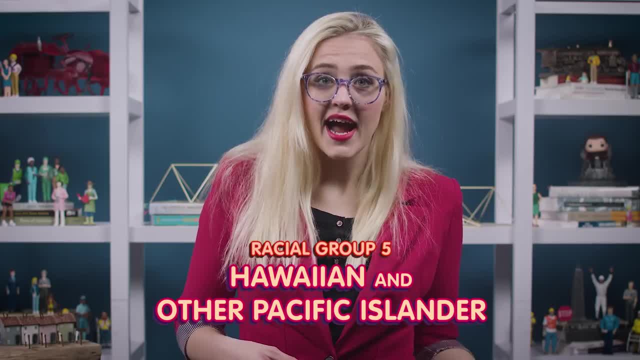 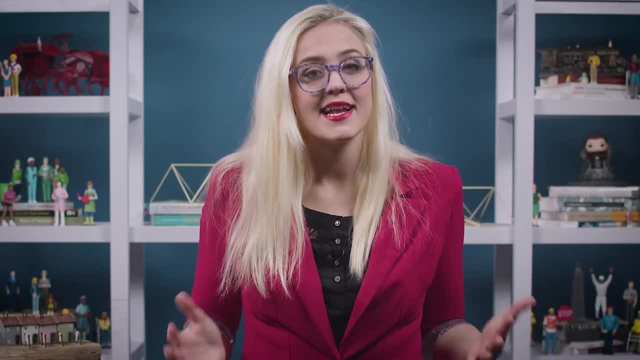 people whose origins are from Hawaii, Guam, Samoa or other Pacific Islands. As I mentioned before, Hawaii is one of the states where a minority race is the majority race for the state and, in fact, it's the only state that has always been minority-majority. 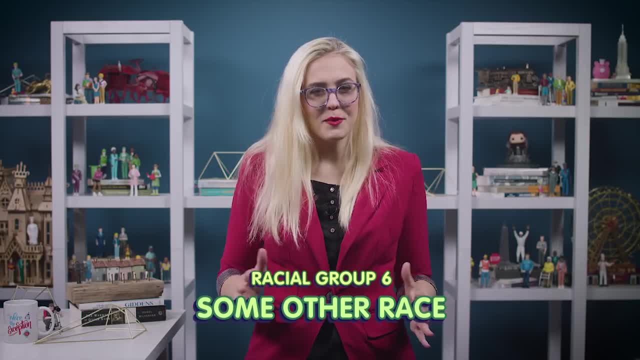 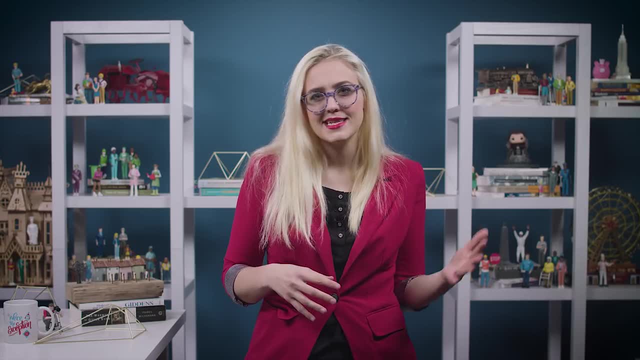 The last census category is just a catch-all- some other race. You might remember that about a third of Hispanic Americans fall into this group. If a person lists a country of origin that doesn't fit in one of the other categories, they get stuck in this group. You might be thinking that these categories don't seem like the racial groups you typically think of, And that's okay. In all likelihood, the way that the government defines races will continue to change to incorporate our society's changing notions of race and ethnicity. 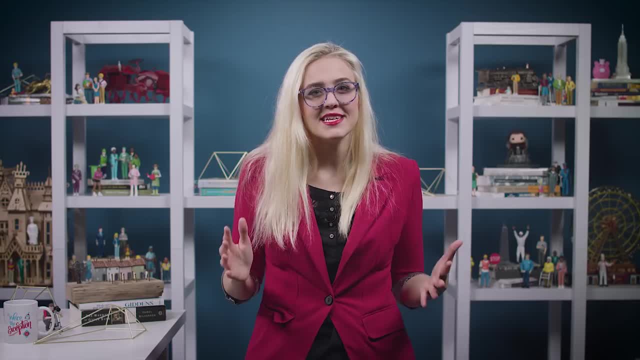 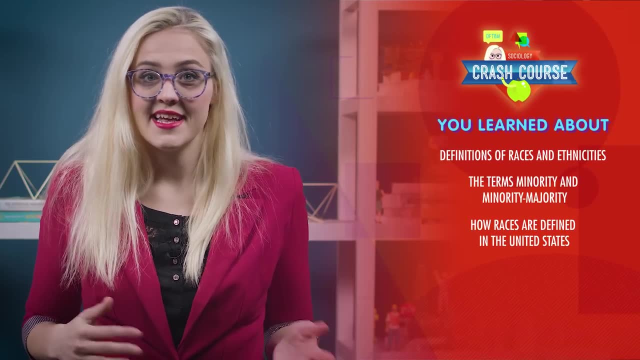 And something that should be clear from everything we talked about today is that races aren't fixed, immutable categories. They are defined by societies. Today, we learned the difference between races and ethnicities. we discussed how definitions of races and ethnicities have changed over time and across places. we also discussed